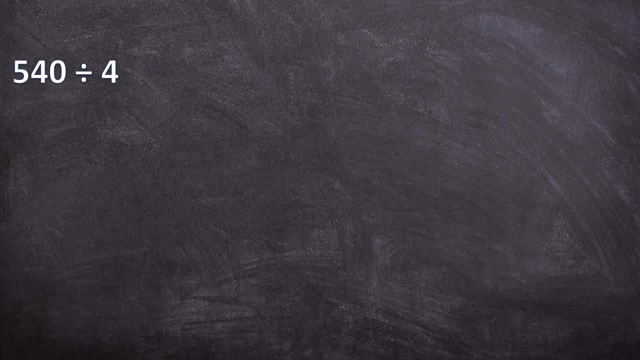 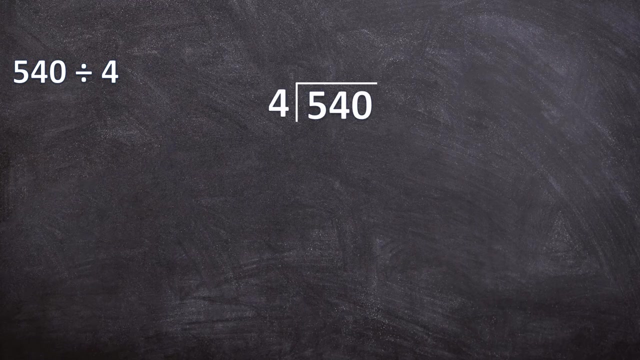 how we're going to write this in the correct format that we can do: our long division. so the first thing we need is our long division bracket. okay, now we take the dividend and we write it underneath the bracket and the divisor goes in front of the bracket. our answer, our quotient, will go on top of the bracket. 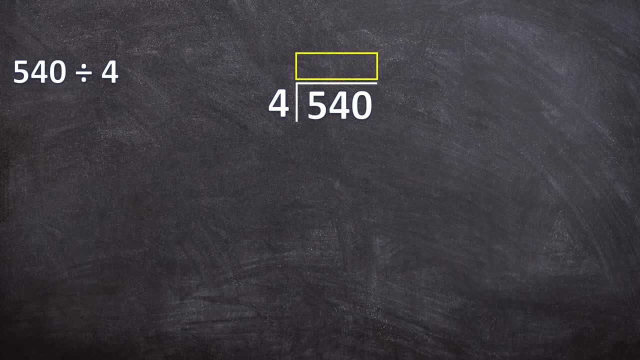 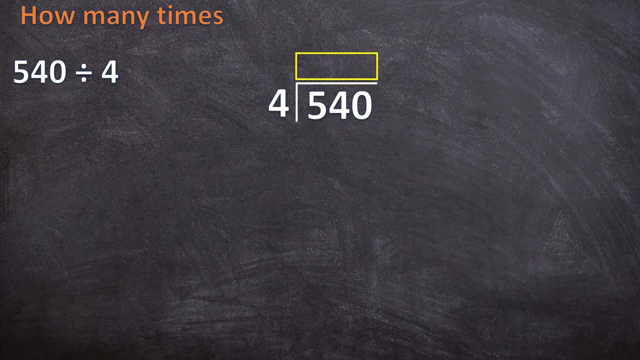 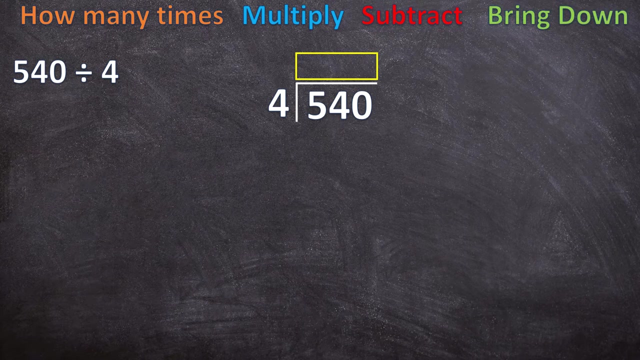 so when you are completing long division, there are four steps. i want you to remember: the first one, how many times. the second one, multiply. the third one, subtract. and the fourth one, bring down. and then, when you're done with bring down, we start all over again from the beginning. 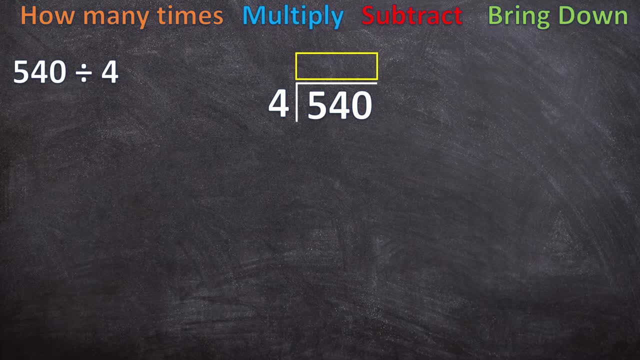 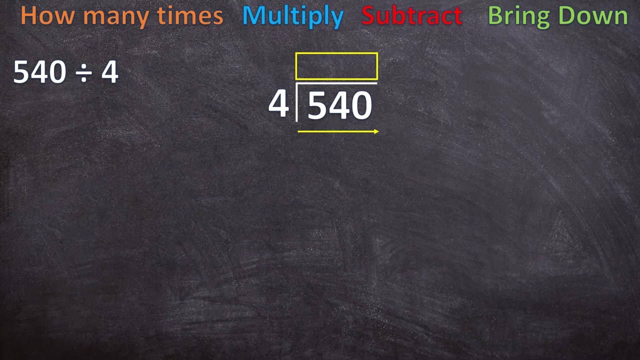 i know this seems complicated now, but you will soon understand what i'm talking about. and the last thing i want you to remember is when we're doing long division, we complete it from left to right. you will now understand what i'm saying, so let's start. okay, so we start with our first step. 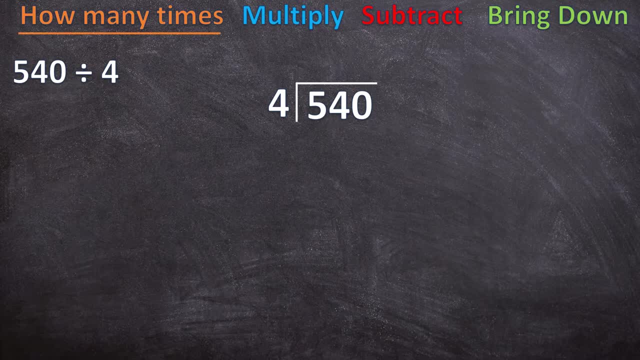 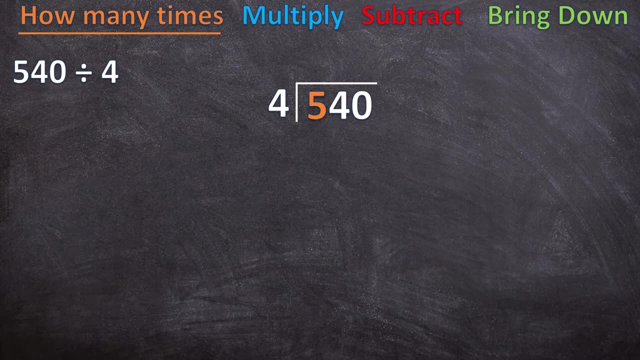 how many times? and, like i said, we go from left to right. so we start with five. now we say how many times can four go into five one time? so our answer goes at the top, at the top of five, not just somewhere randomly, just a bit of time. 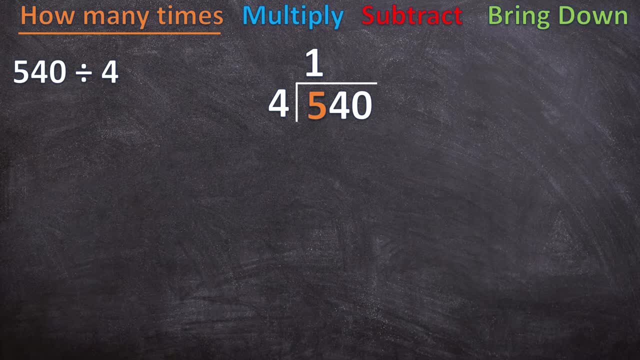 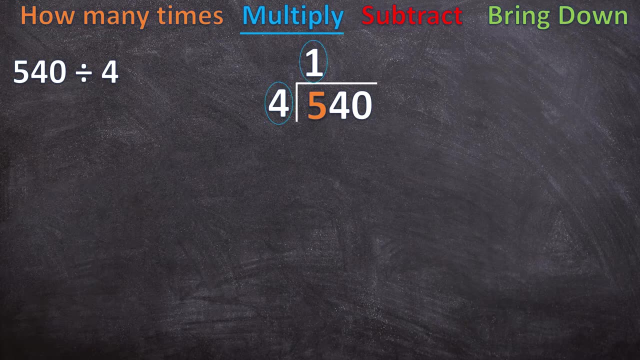 5.. Now we move on to the next step: multiply. Now we say what is 1 times 4, and 1 times 4 is 4.. We write that exactly at the bottom of 5, not just somewhere randomly exactly beneath 5.. Now we move. 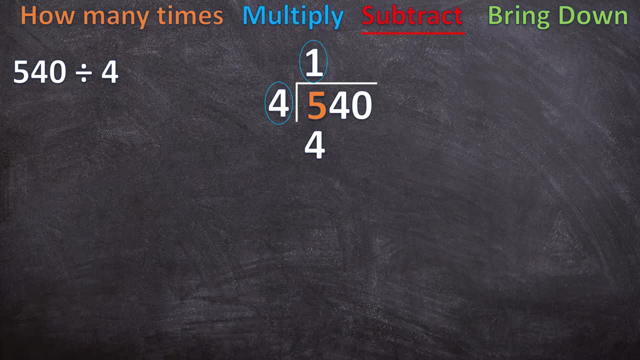 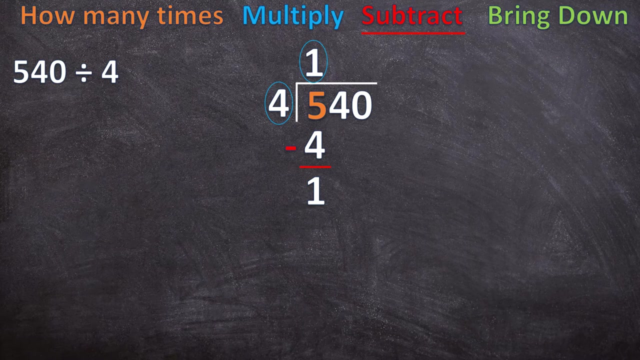 on to the next step. subtract. Now we say what is 5 minus 4.. 5 minus 4 is 1, and now the last thing we do is we move on to the next number. like I said, we go from left to right. the next one is 4 and we 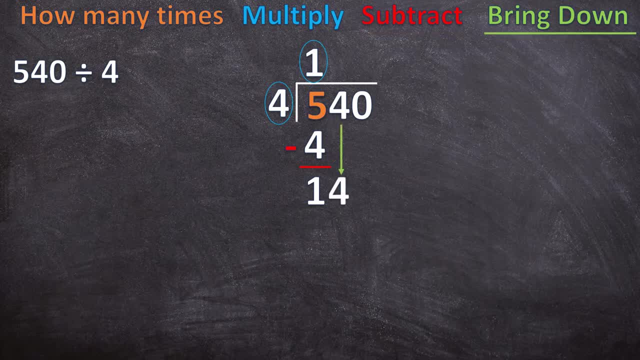 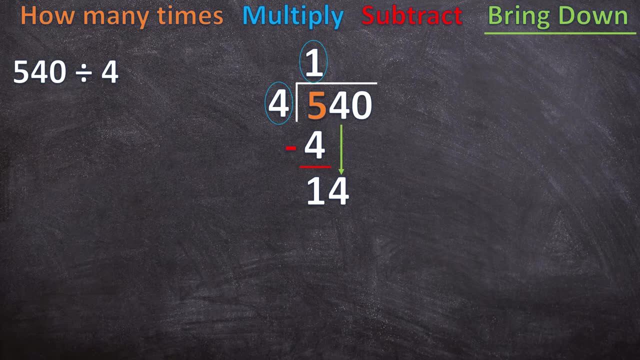 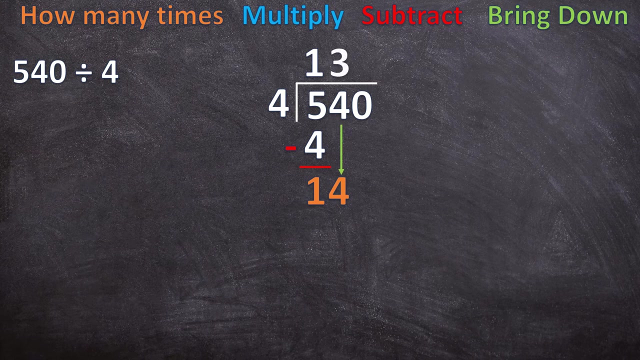 bring the 4 down. Now that you've done that, you start all over again. So what's the first step? So how many times can 4 go into 14? 4 can go into 14 three whole times. Now what's the next step? The next step is: multiply. So 3 times 4 is 12.. The next step: 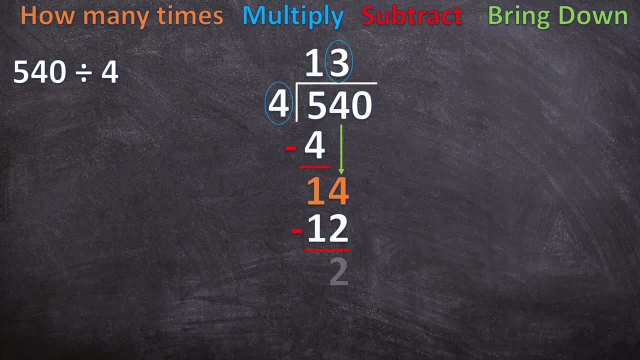 subtract 14 minus 12 is 2.. The last tip: bring down the next one. So what's the first step? So how many times can 4 go into 14?? 4 can go into 14 three whole times Now. 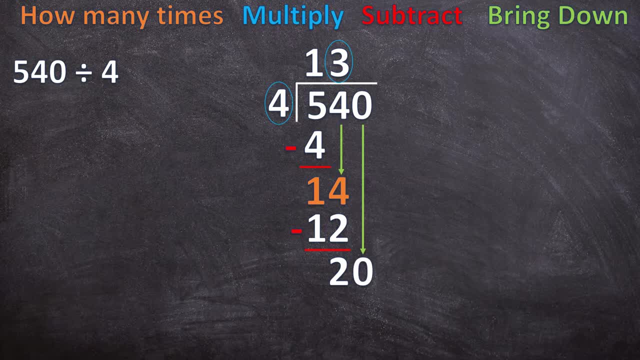 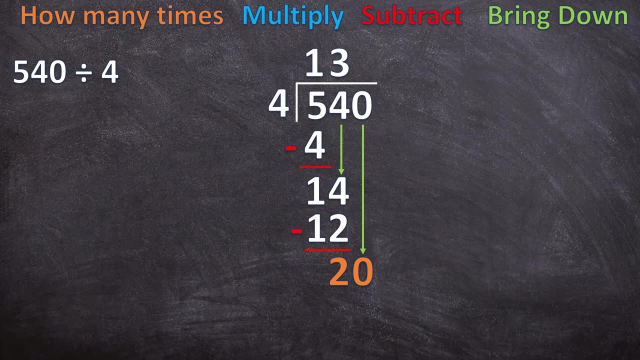 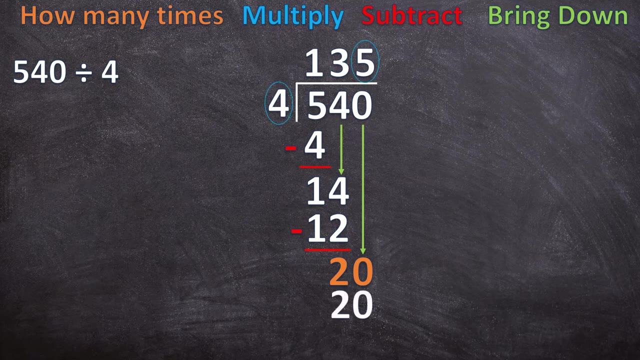 the next one is 0.. So we bring that down. Now we start all over again. How many times can 4 go into 20? 5 times, 5 times 4 is 20, and 20 minus 20 is 0.. There's nothing else to bring down, and there is. 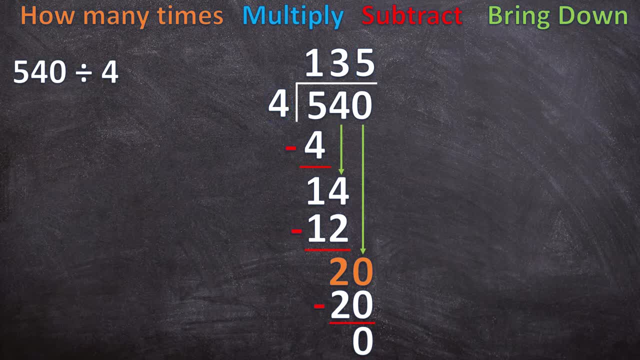 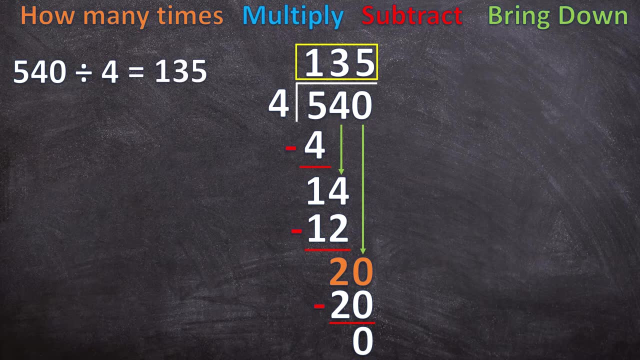 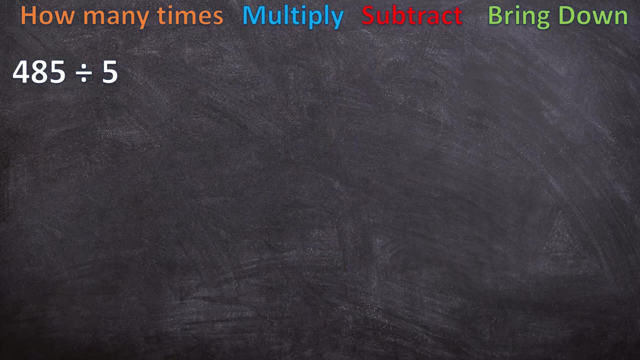 no remainder, We end it with 0.. So the final answer is 135.. So now let's go on to the next example. Now, this example is slightly different, and you'll see now why I say so- but it doesn't matter how different it is: We follow the exact same steps in the exact same way. 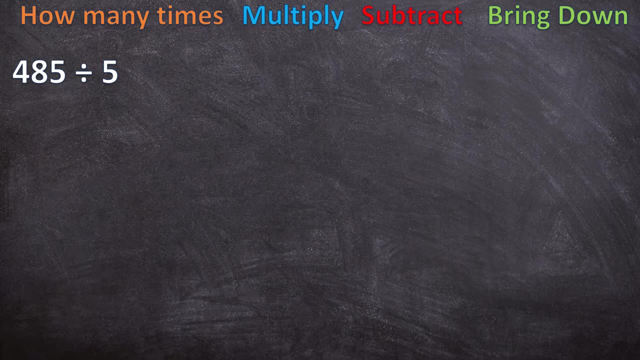 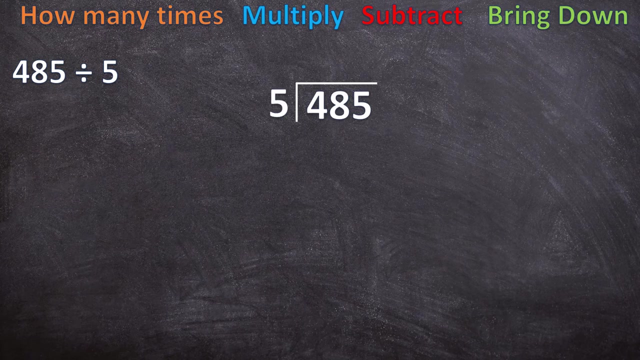 We never change our steps. So if you just follow those steps, you will get at the correct answer. So the first thing we do is we write down our long division brackets and then our dividends goes inside and our divisor goes in front of the brackets. So now we start again from left to 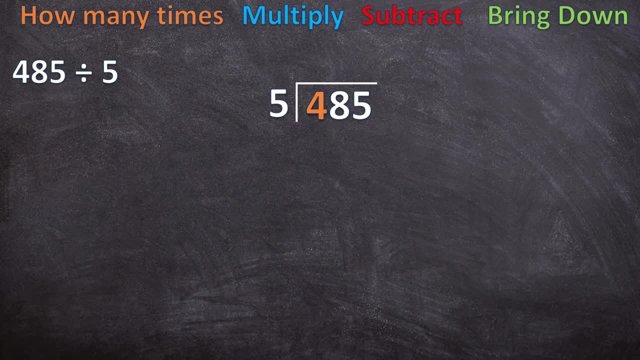 right. We say: can 5 go into 4?? No, 5 cannot go into 4.. So just to visualize that for myself to remember. So we take the next step and we are going to work this out. So let's go ahead and let's. 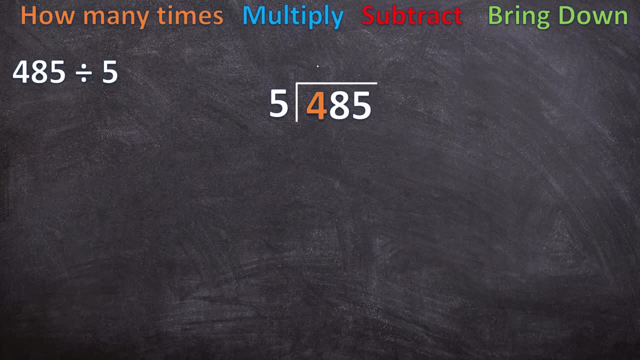 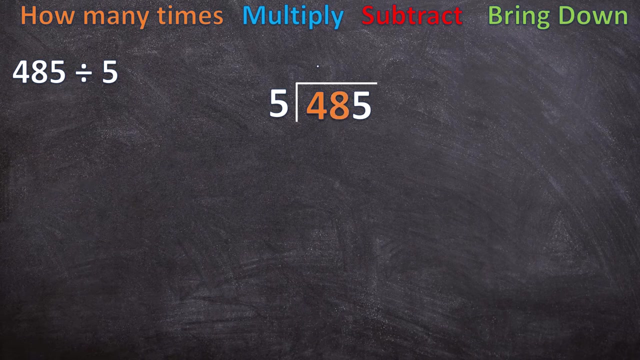 I'm just adding a dot there so that I know: okay, now five cannot go into four. so I'm leaving the space above the four open. there must be nothing now. I move on to the next one. I now say: can five go into 48? yes, five can go into 48. how many times? nine times, and now I multiply nine times five. 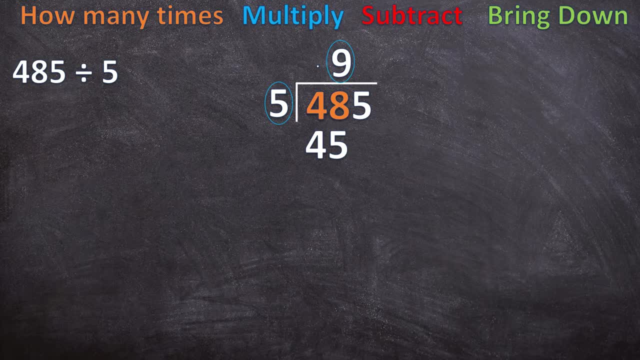 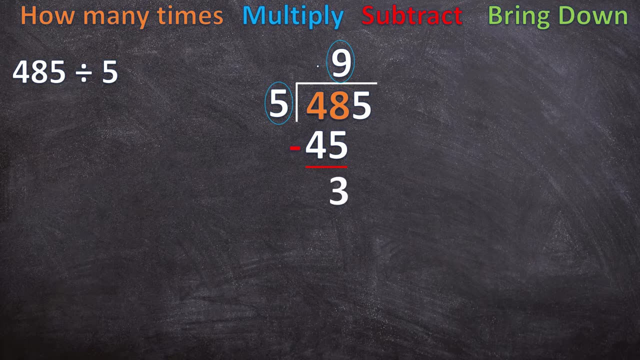 is 45, then I follow my steps, then I subtract: 48 minus 45 is three, and then I bring down the five. so now what's the next step? we start all over again. so can five go into 35? yes, how many times? seven times. and now the next step. 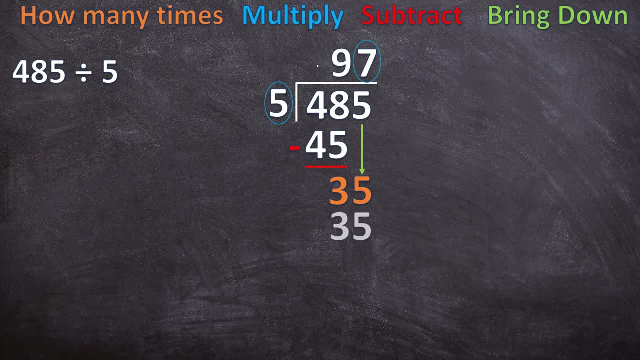 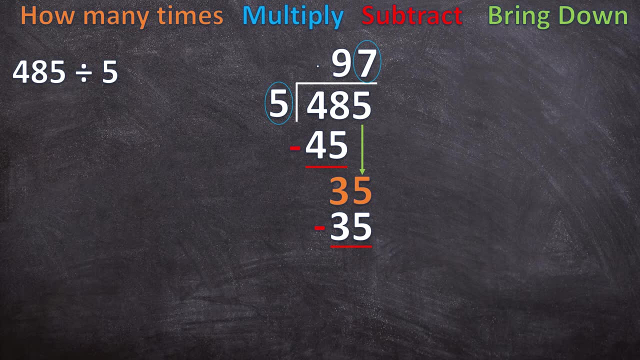 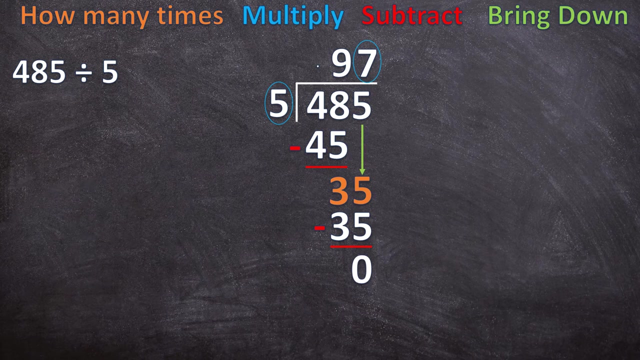 seven times five is 35. and now in the next step, we subtract. so what's 35 minus 35? that will be zero. there's nothing else to bring down, and we ended at a zero, so there's no remainder. so our answer is nine seven. now let's look at this last example, again slightly different, but you'll now see what I mean. 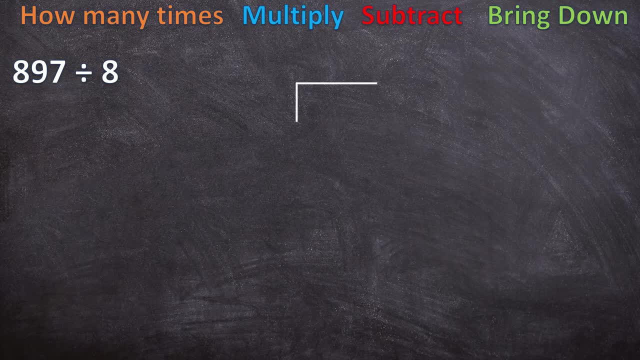 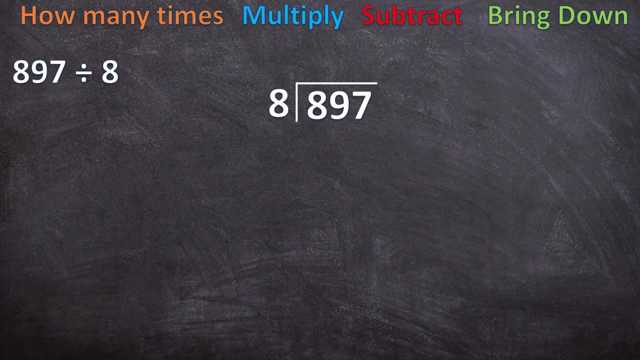 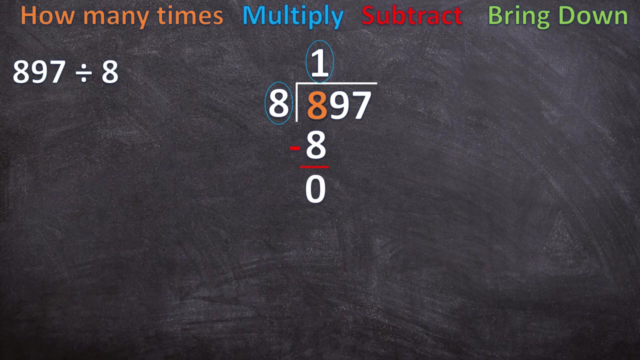 by that. so first we write down our long division, bracket 897 underneath the bracket and the eight in front of the bracket, and now we start calculating: can eight go into eight? yes, it can. how many times once? and now we multiply one times eight is eight, and we subtract: eight minus eight is zero. so now we bring down the next one. so we bring down the nine, and now we start at the first step again. how many times, how many times can eight go into nine? and that is one time and one times eight is eight. now we subtract: nine minus eight is zero. so now we bring down the next one. so we bring down the nine. and now we start at the first step again. how many times, how many times can eight go into nine? and that is one time and one times eight is eight. now we subtract: nine minus eight is zero. so now we bring down the next one. so we bring down the nine, and now we start at the first step again. how many times, how many times can eight go into nine? and that is one time and one times eight is eight. now we subtract: nine minus eight is zero. so now we bring down the next one. so we bring down the nine and now we start at the first step again. how many times, how many times can eight go into nine? and that is one time. and one times eight is eight. now we